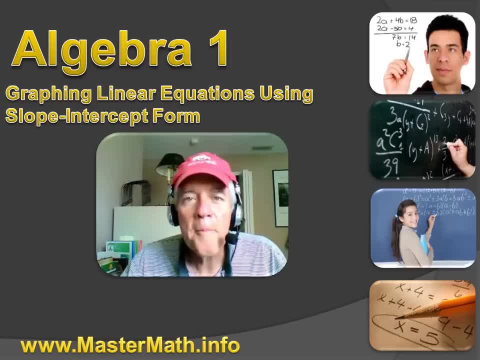 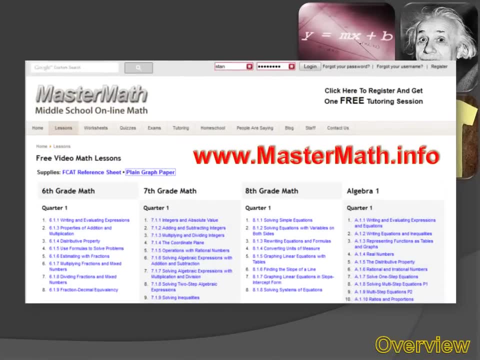 I hope you have a really good time today. Welcome to our lesson on graphing linear equations in slope-intercept form. You're going to need some graph paper. If you don't have any handy, go to my website, wwwmastermathinfo. 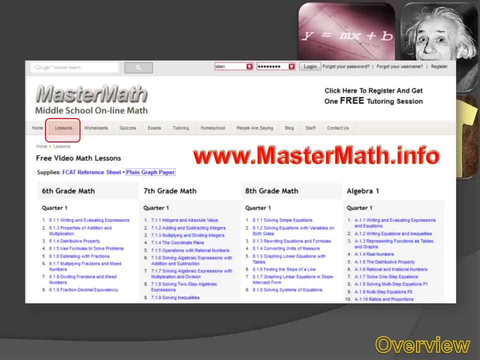 and then hit the Lessons tab On the Lessons page. you'll see a link right about there to the lesson. If you don't have any handy, go to my website, wwwmastermathinfo, for plain graph paper. If you click on that link, a sheet of graph paper will suddenly. 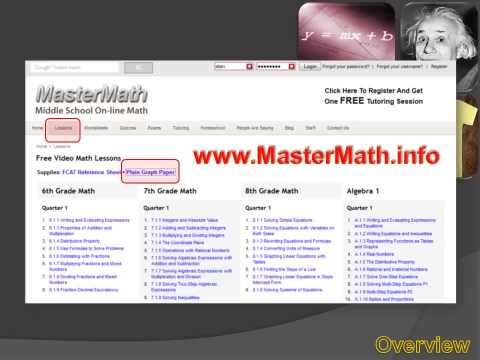 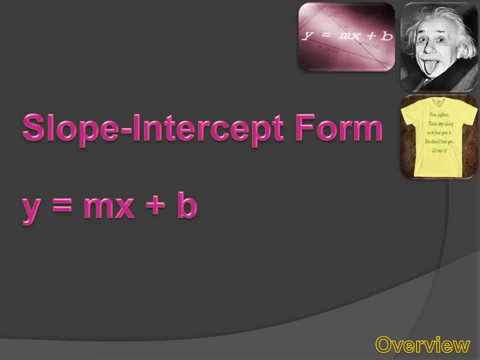 appear and you can print that and use it during this lesson. During this lesson, we're going to be talking about slope-intercept form, which is y equals mx plus b, and we're also going to talk about parallel lines. Now, hopefully by now you know how to do. 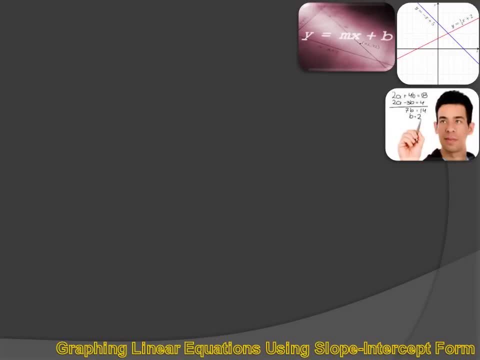 this. You know how to graph a linear equation using tables and using the intercepts, But today we're going to learn about the big kahuna. y equals mx plus b. When you get comfortable with y equals mx plus b, you'll probably. 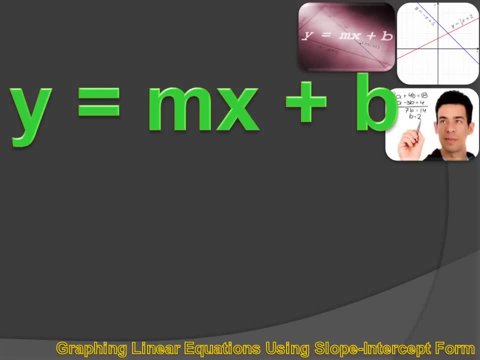 never graph using intercepts again in your life. Well, what does y equals, mx plus b mean? I mean, I can see there's a couple of variables in there. I can see there's a y and I can see that there's an x. but what's that m mean and what's that b mean? Well, 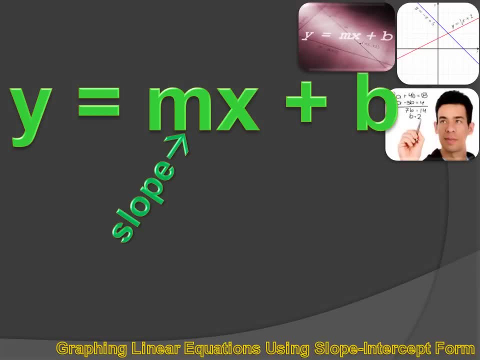 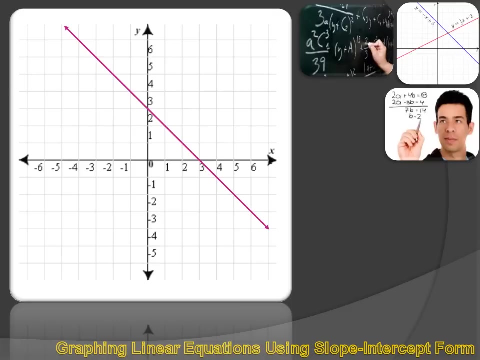 guess what I'm going to tell you. The m is the slope of the line and the b is the y-intercept. If I know the y-intercept and I know the slope of the line, I'm going to graph it. I can graph it. Maybe it makes sense to review slope and intercept real. 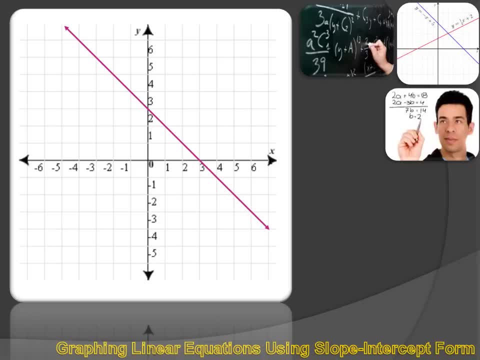 quickly before we go any further into this lesson. What is slope? Well, hopefully you remember that slope is rise over run. I take any two points on the line and I find out how much I rise and how much I run in order to get from the first point to the second. 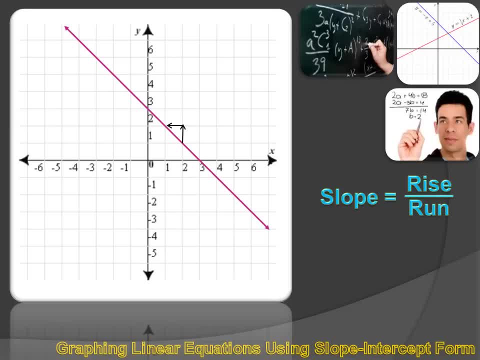 point To make that division rise, divided by run, I'll know the slope of the line. For instance, on this line I rise positive one and I run negative one, so my slope is one over negative one or a slope of negative one. How about intercepts? What do intercepts mean? Well, 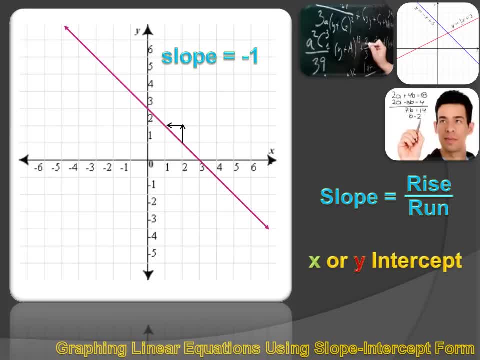 there can be either an x-intercept or a y-intercept. That's just where the line crosses the x or the y-axis. You can see that green circle. Well, that's where the line crosses the x-axis and that's the x-intercept. And the red circle 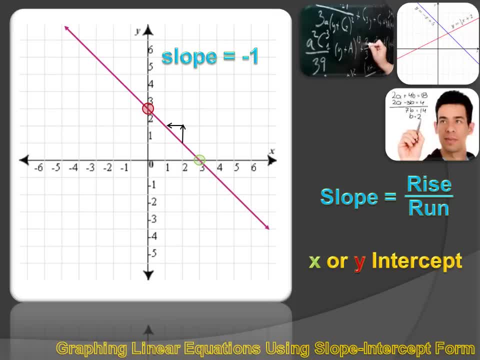 is over the point where the line crosses the y-axis and that's the y-intercept. So this line has a slope of negative one and a y-intercept of two, And you need to memorize this formula: y equals mx plus b. That m stands for the slope. 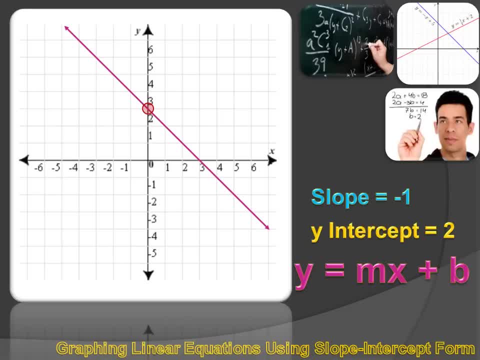 of the line, And if I replace that m with the actual slope of the line minus one, then my equation becomes: y equals minus one, x plus b, b. What's b mean? Well, b is the y-intercept, And in this case our y-intercept is negative one. So that's the y-intercept. 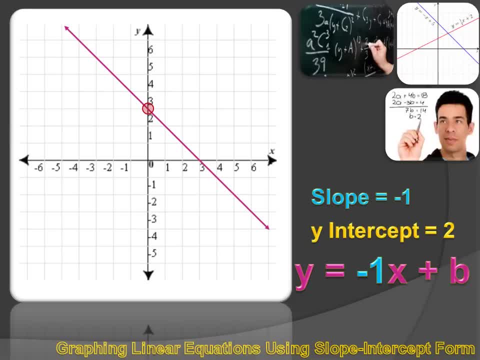 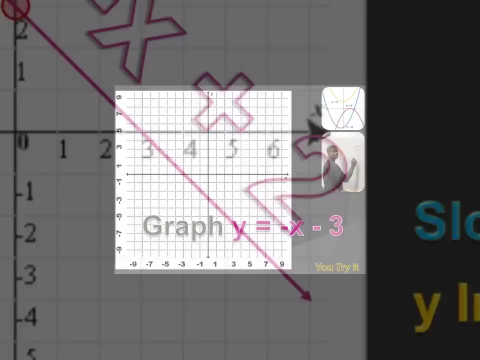 The y-intercept is two. So if I replace that b with the positive two, my equation becomes: y equals minus one, x plus two. So the equation for this line is y equals minus x plus two. Here's one for you to try, But if you don't get it, don't worry about it. 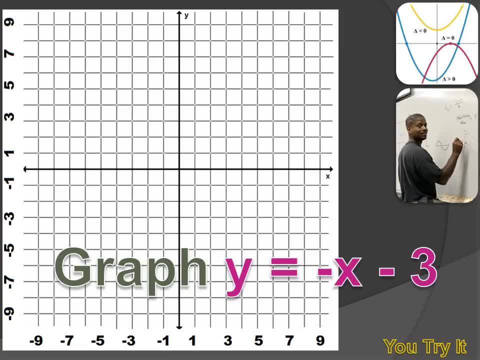 This is a little tough. I want to see if you can figure this out, though I want you to graph. y equals minus x, minus three. Now you remember that I've got that in slope-intercept form, So my slope is that minus or minus one, And my y-intercept is minus three. So if I start with one point, 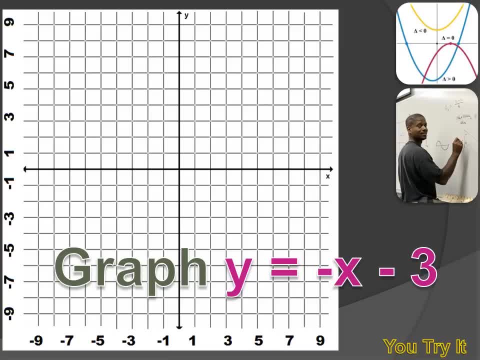 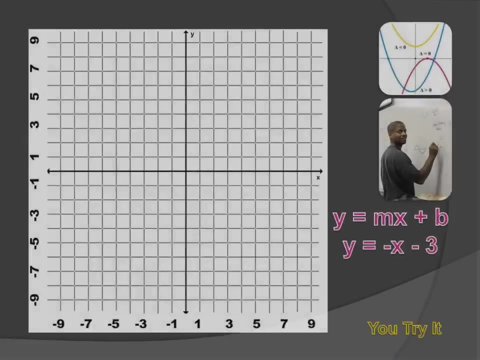 on the graph and use the slope to figure out a second point on the graph. I'll have two points and then I can graph the equation. You try it, Hit your pause button, try the problem and then hit the forward key to move on to the answer. 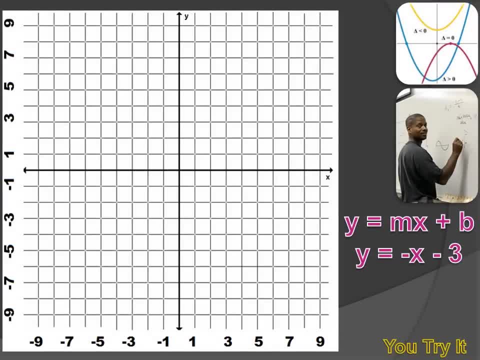 Did you get it? I hope so. Hopefully you remember that y equals mx plus b is the standard form for a slope-intercept. b is the standard form for a slope-intercept. b is the standard form for a slope-intercept. 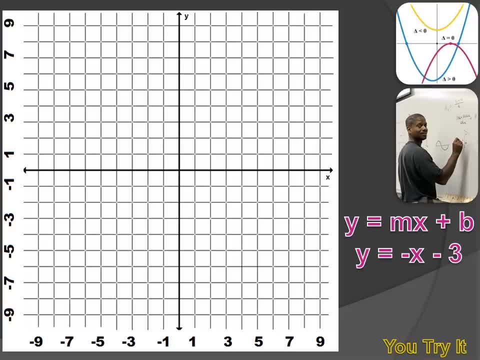 And the m equals the slope and the b equals the y-intercept. Well, our equation is: y equals minus x, minus three. So what would b be? What would the y-intercept be? Well, it would have to be minus three. So we can identify one point on the line by identifying the y-intercept. 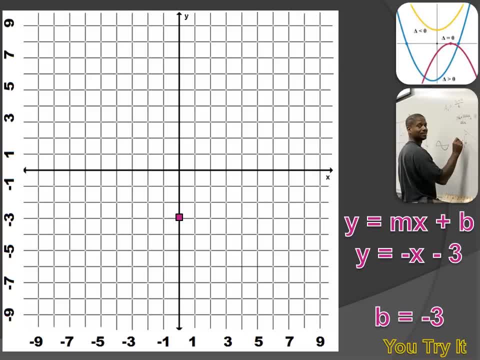 Okay, So we can find where the y-intercept is at minus three. Now we've got one point, but we haven't used our slope yet, And the slope of this line is minus one, A slope of minus one. Well, you remember, slope equals rise over run. So I need a ratio or a fraction. 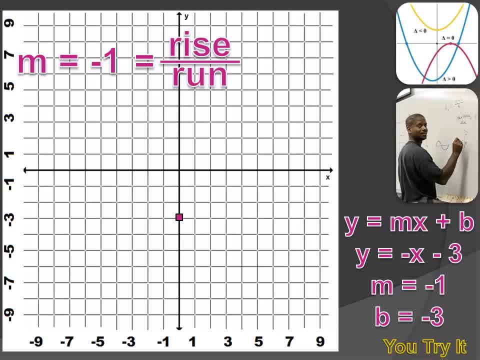 that equals minus one. I need to convert minus one to minus one. I need to convert minus one into one of the many, many combinations of rise over run that equals minus one, And one of those combinations would be a rise of minus one and a run of positive one. But 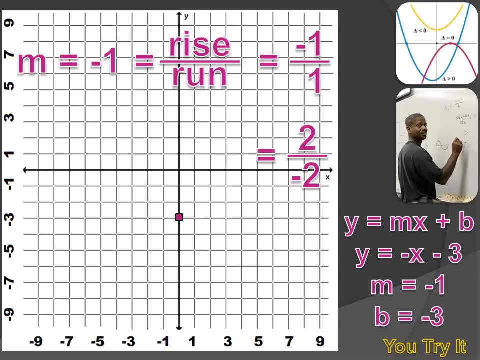 that's not the only one that works. We could also have a rise of positive two and a run of negative two, because positive two over negative two equals minus one, just as minus one over positive one equals minus one, So you could use any fraction that equals minus. 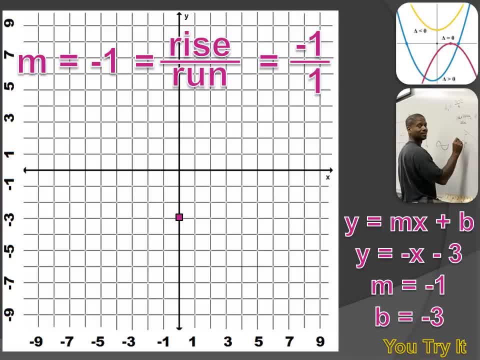 one. I'm going to use minus one over positive one, because that just seems like the easiest one. So I've got a rise of minus one, So I'm going to go down one. from my starting point, I'm going to go down one, And then I've got a run of positive one, So I'm going 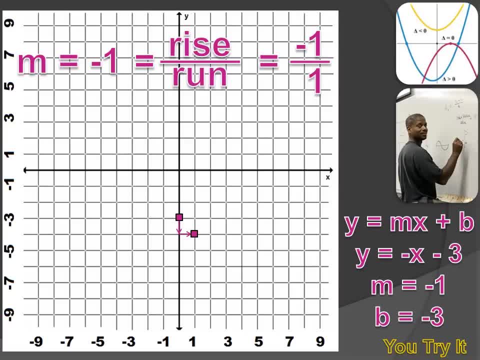 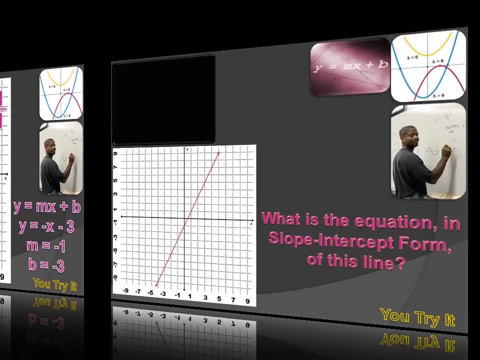 to go one to the right And that identifies a second point on my line. Now I've got two points. It's a simple matter to run a line through them, And that is the line that represents the equation: y equals minus x minus three. 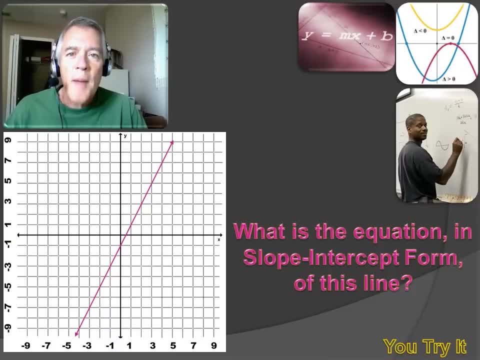 Now you try this one: Hit the pause button, do the problem and then hit the forward key to move on to the answer. Well, in order to figure out what the equation to this line is, I need two bits of information: I need to know what the slope of the line is and I need to know what the y-intercept. 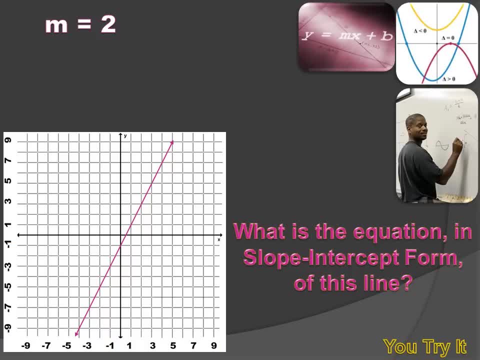 is: Let's figure out the slope first. The slope equals two. How do I know that? Well, I'm going to go down one from my starting point and then hit the pause button, do the problem and then hit the forward key. So I pick any point on the line And I want to. 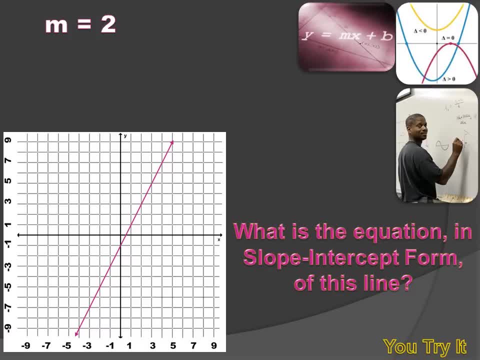 pick a point where I've got x and y axis lines that intersect, And I'll pick that point right there. And then I have to pick a second point And I'm going to once again look for a point where my x and y axis lines intersect And I'll pick that point right there. Then 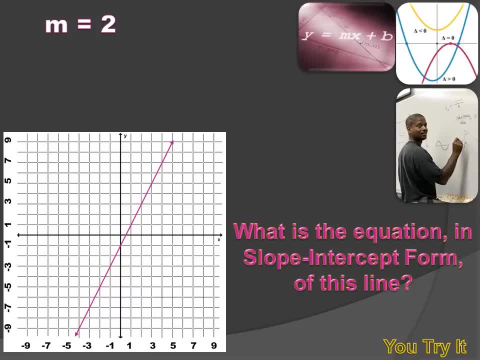 I figure out my rise. one two over my run. one Two over one equals a slope of two. Now I've got to figure out what the slope of the line is. I'm going to go down one to the right. 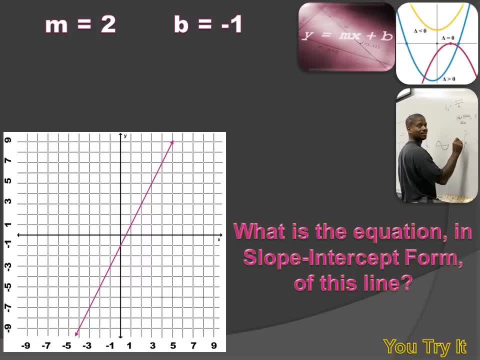 Let's figure out what my y-intercept is. Well, my y-intercept is minus one. Where does this line cross the y-axis? Right there, at minus one. So now I know my slope is two and my y-intercept is minus one. And the basic form for an equation in slope-intercept form is: 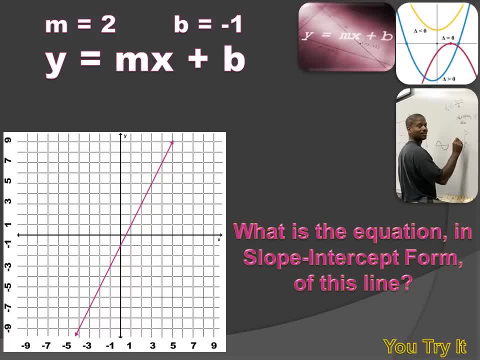 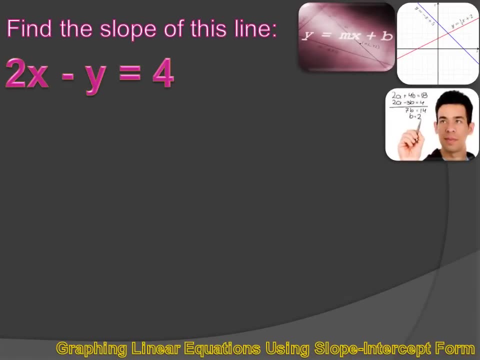 y equals mx plus b. I just substitute two for mx and I get y equals mx plus b And this line's equation is: y equals 2x minus one. Well, what if they gave you an equation like this: 2x minus y equals four, And they said: find the slope of this line, Could you? 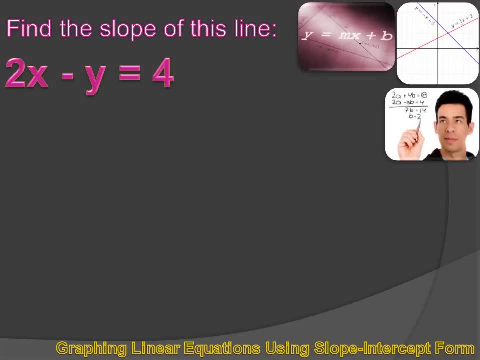 do it? Yeah, you could, But first you're going to have to manipulate this equation a little bit. You're going to have to move it around, change it about until it's in the form: y equals mx plus b, And you're good enough at algebra to do that. I think the 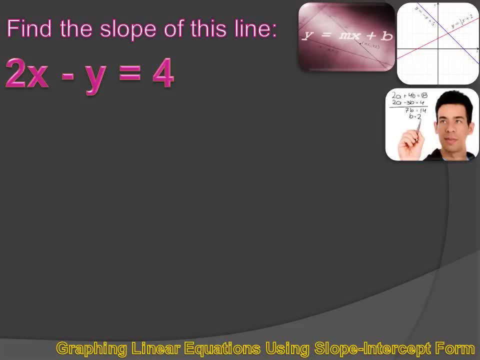 first thing I want to do is put my negative y on the right side of the equation, so it's no longer a negative y. So I'm going to add y to both the left and the right side of the equation And now it's going to read: 2x equals four plus y. Now I've got to isolate that. 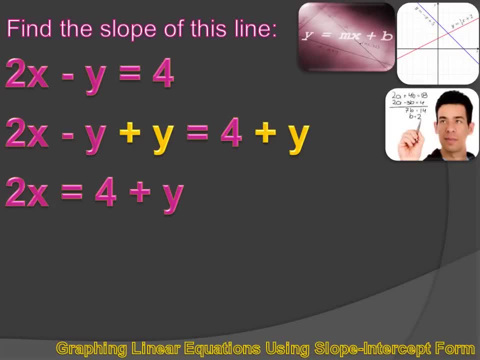 negative y. So I want to move that four to the left side of the equation, which means I've got to subtract four from both the right and the left side of the equation And now the equation reads: 2x minus four equals y. Well, hopefully you can see that's slope intercept. 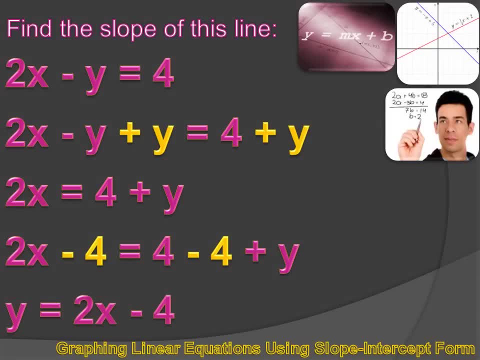 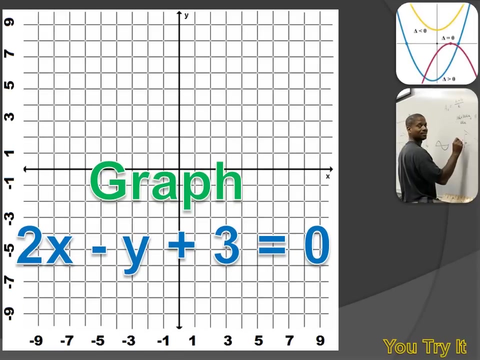 form. But if you'd like to be completely regular about it, we can turn it around so it reads: y equals 2x minus four. That's slope intercept form, And my m is two, So my slope is two. Try this one. Hit your pause button, graph this equation and then hit your forward key. 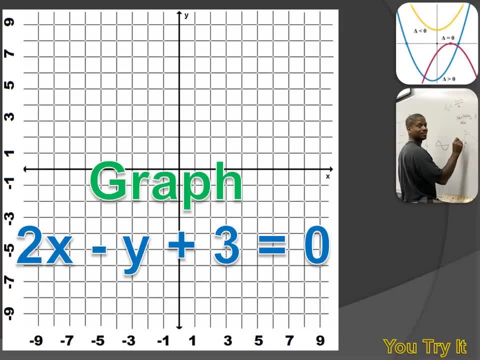 to move on to my answer. Well, it's easy, I hope you see, to graph an equation that's in slope and intercept form. But this equation isn't in slope intercept form, So I'm going to have to manipulate it. So I'm going to have to manipulate it, So I'm going to have. 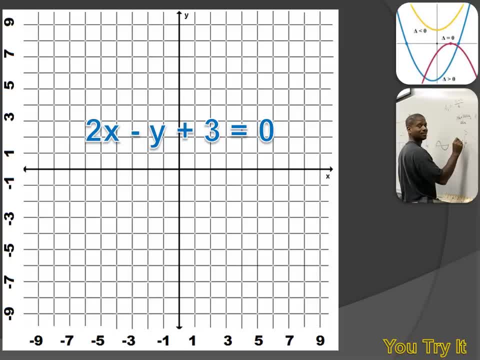 to manipulate it a little bit. Seems to me that the easiest way to get this into slope intercept form is to take that negative y and move it to the right side of the equation so it becomes positive y, And then I've got y equals something. So let's do that. I'm 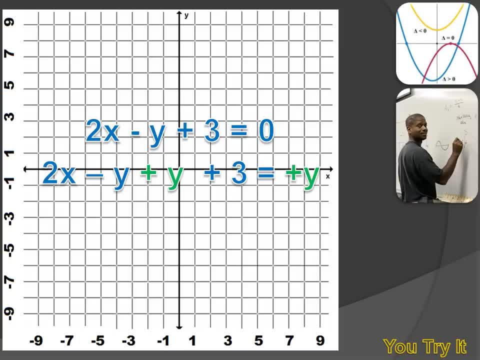 going to add y to both sides of the equation. On the left, the y's cancel each other out And on the right, I'm left with a positive y And my equation reads: 2x plus 3 equals y, Which hopefully you understand, is the same thing as y equals. 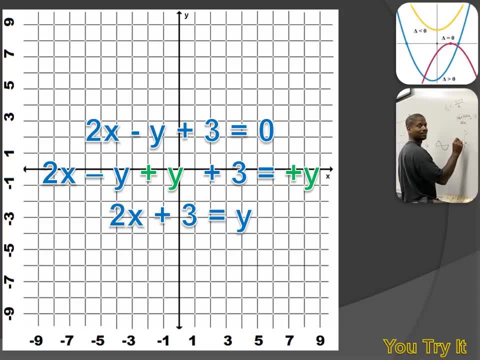 2x plus 3.. And now I know my slope 2, and I know my y-intercept plus 3.. So now I can graph it. First let's identify that y-intercept positive 3.. Now my slope is positive 2, a. 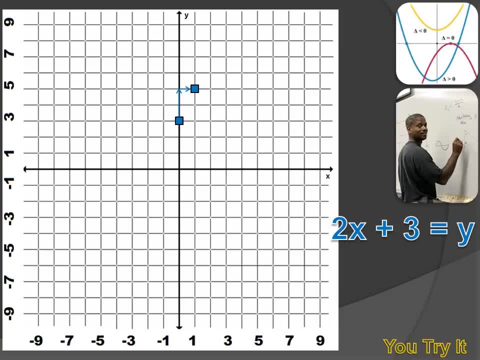 rise of 2 and a run of 1.. So I'm going to add y to both sides of the equation, And now I know my slope: 2, and a run of 1.. So now I can plot a second point, And if I've 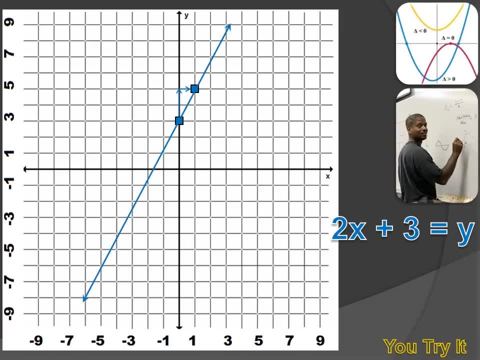 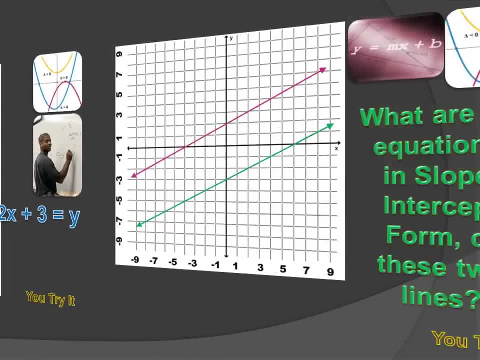 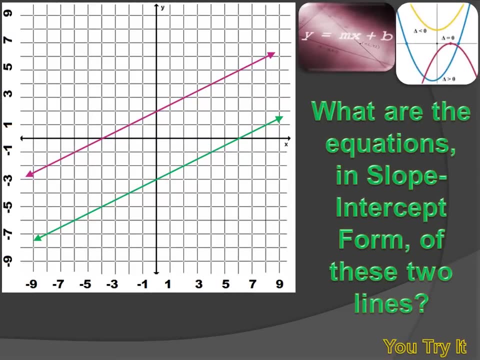 got two points. I can draw a line, And that is the line for y equals 2x plus 3.. You try this one. Determine the equation in slope-intercept form for the purple line and the green line And then look at those two equations and tell me what you think about. 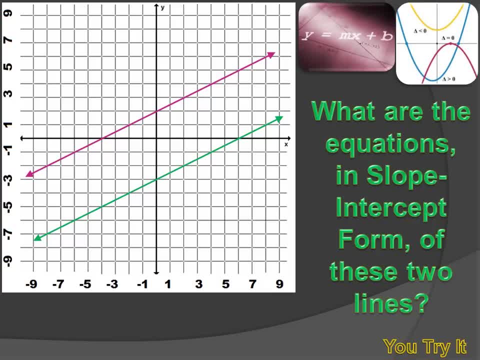 them. Hit your pause button, try the problem and then hit your forward key to move on to my answer. Well, let's get the equation of the purple line first. We're going to need to get the slope and the y-intercept. Well, the slope would be a rise of 2 positive and 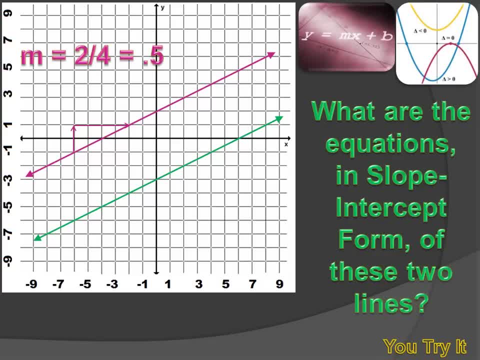 a run of 4 positive. So my slope is 2 over 4, or one-half, or 0.5.. What's my y-intercept? Well, it's right there. It crosses the y-axis at 2.. So my y-intercept is 2.. Now, if I've 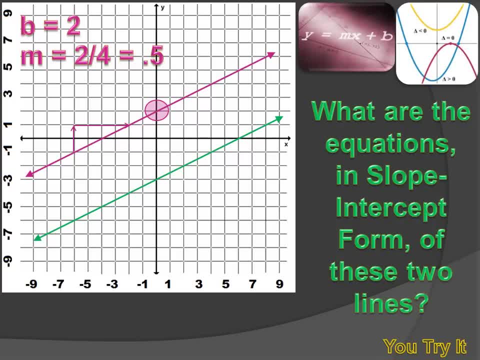 got my slope 0.5, and I've got my y-intercept 2,. I can write the equation, which would be: y equals 0.5x plus 2.. How about the green line? The green line and the purple line are parallel lines, aren't? 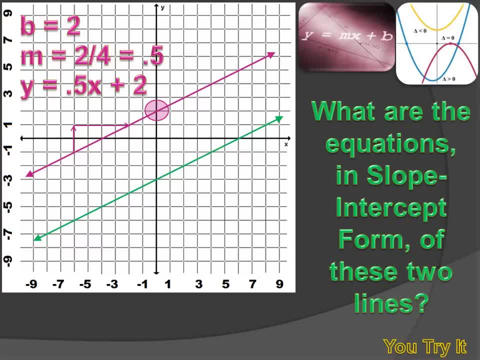 they. They look like they're exactly the same distance apart everywhere you go. I wonder what that's going to mean in terms of their equations. Well, let's take a look. First let's calculate the slope, And again I have a rise of positive 2 and a run of positive. 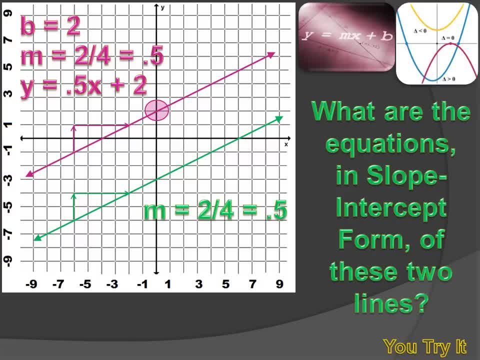